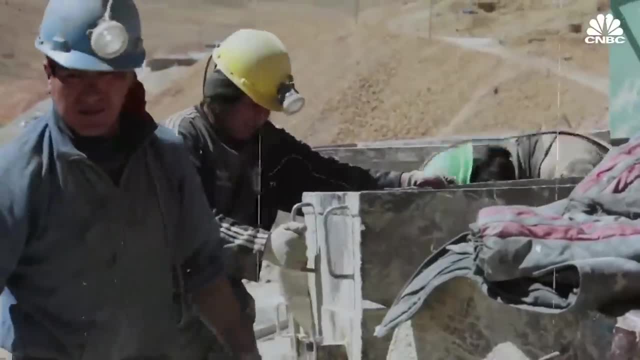 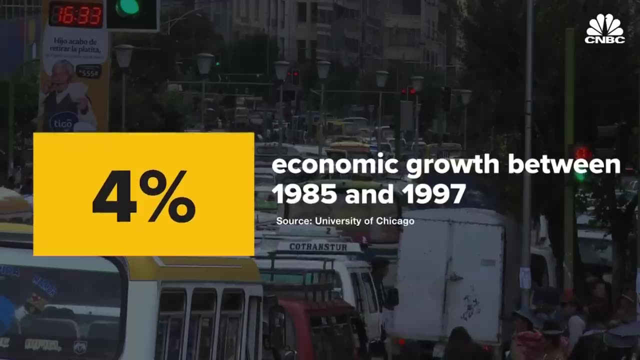 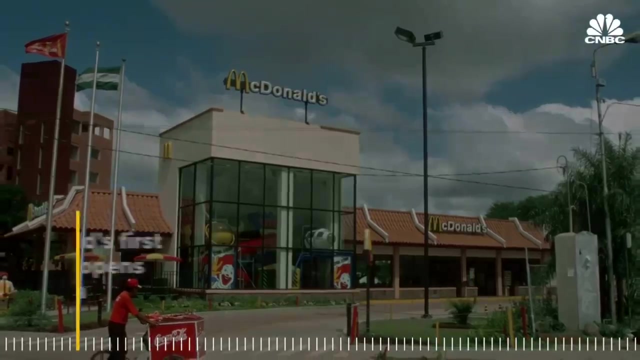 foreign investors. By the mid-90s, international companies began to flood the market, which ultimately played a role in helping rev up Bolivia's economy. On average, the economy grew 4% between 1985 and 1997.. That's when McDonald's entered Bolivia. The first Bolivian location opened. 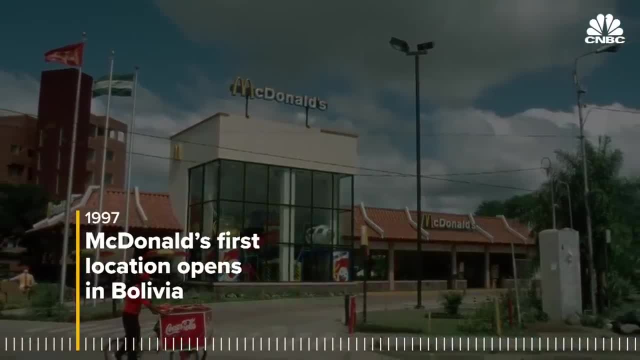 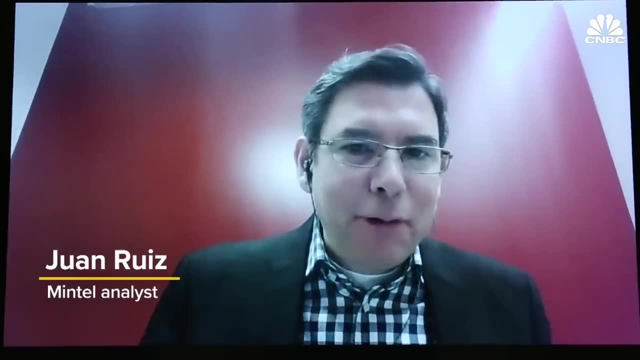 its doors to the public in 1997 in the city of La Paz, And it was met with a lot of hype. It was like huge social event. no, You had to go there with your friends, you had to go there with your. 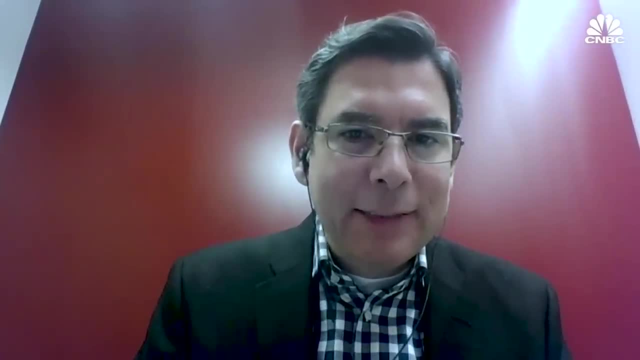 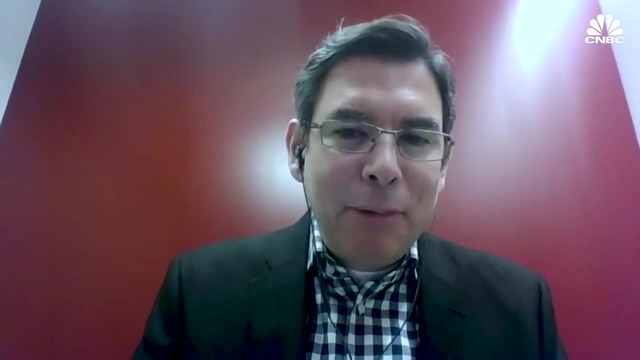 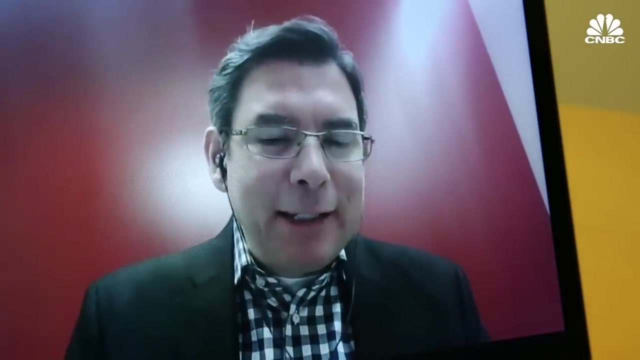 family and people were willing to spend significant amount of time in line just to get there and try And it was interesting because it was a huge line of people standing And then the drive-throughs there were also like a huge line and interrupting all the traffic on the street. 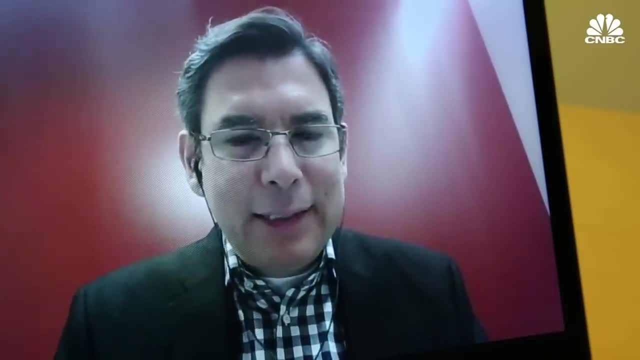 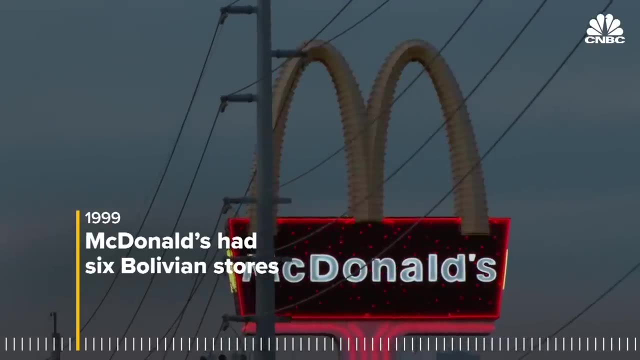 and they're having to go into the side roads and things like that. So it was. it was extraordinary to see By 1999, the American fast food chain had six stores in the country. Its menu was tailored to reflect Bolivian taste buds. McDonald's offered things like: 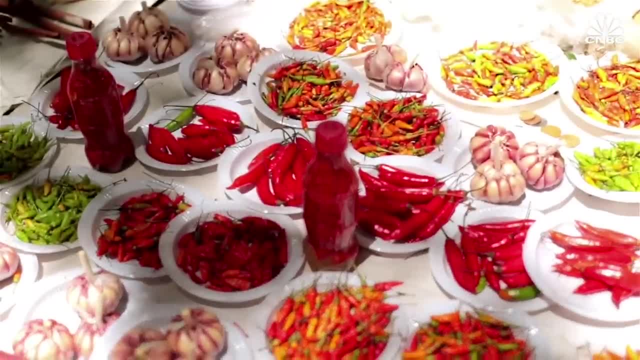 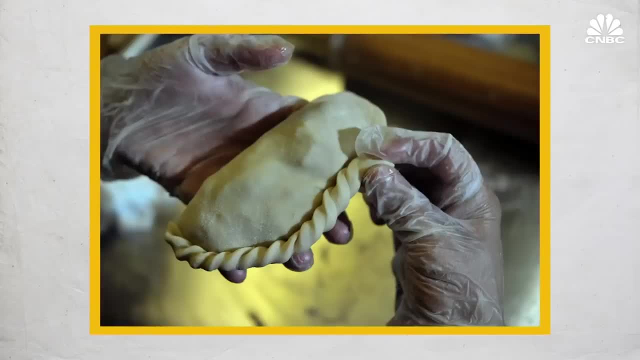 yawa, a Bolivian hot sauce that was made of tomatoes and hot chili peppers. McDonald's even tried to introduce the mixed sultanas, which was a spin on the traditional Bolivian dish known as sultanas. The sultanas are traditional Bolivian empanadas that can. 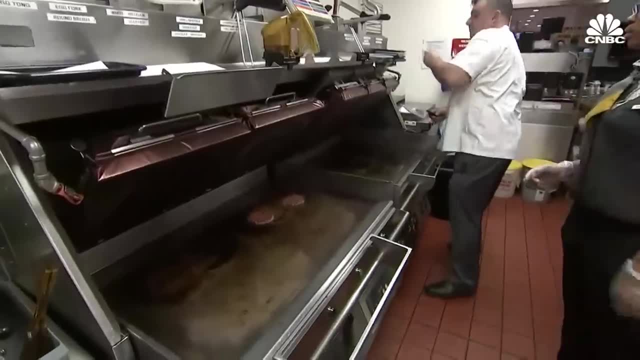 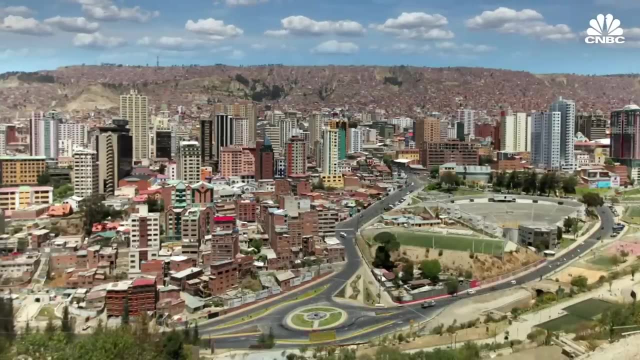 either be filled with savory or sweet foods. but it ultimately did not reach the Bolivian market due to safety standards. But despite McDonald's initial interest from the Bolivian people, lines for McDonald's grew smaller and smaller. By 2002, McDonald's operation in Bolivia expanded to Santa. 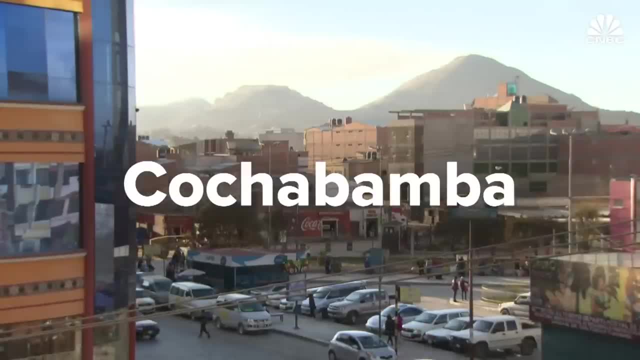 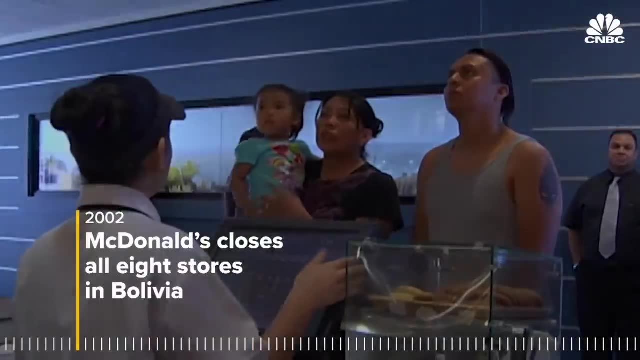 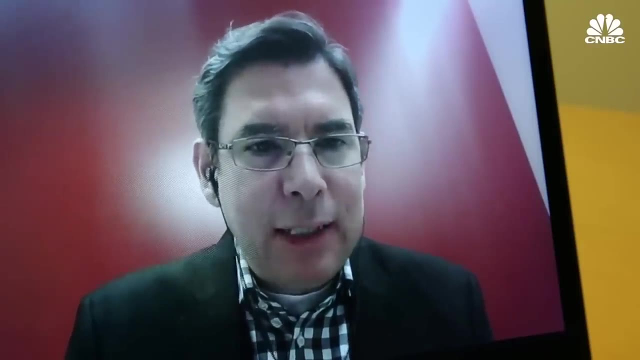 Cruz and Cochabamba in an effort to reach the country's middle-class consumers. But that effort to appeal to Bolivia's middle class failed to shore up sales. In 2002, the American fast food chain shuttered all of its eight stores in Bolivia. It specifically went after the most. 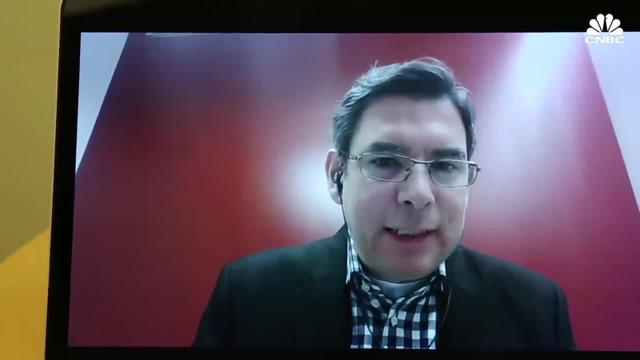 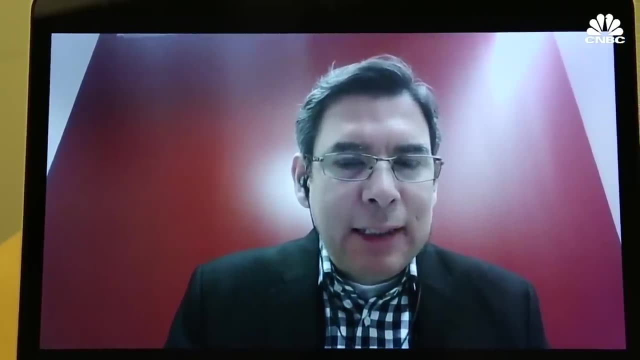 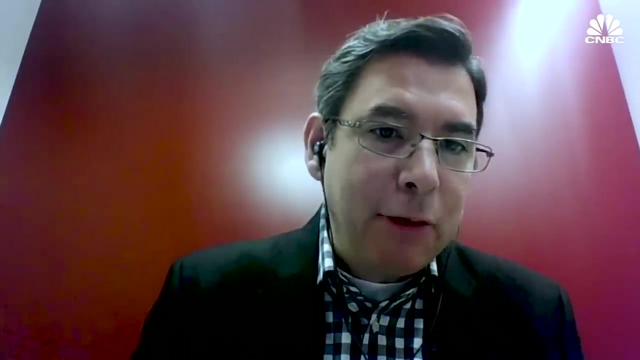 affluent group, So to say. it was an affluent neighborhood in the south side of La Paz. it was in downtown La Paz, so it didn't go really into the areas that are more were more indigenous. Probably that was a second step, but the first step of entering Bolivia was 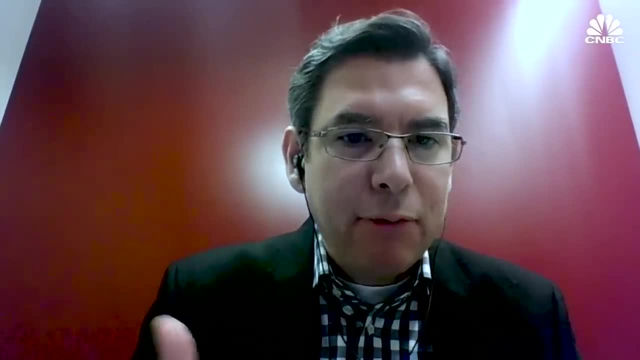 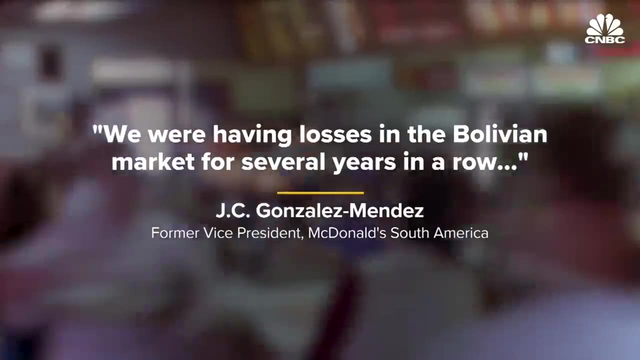 really to appeal to the more affluent people who have, I think, some type of exposure to McDonald's. The former vice president of McDonald's South America said that we were having losses in the Bolivian market for several years in a row. 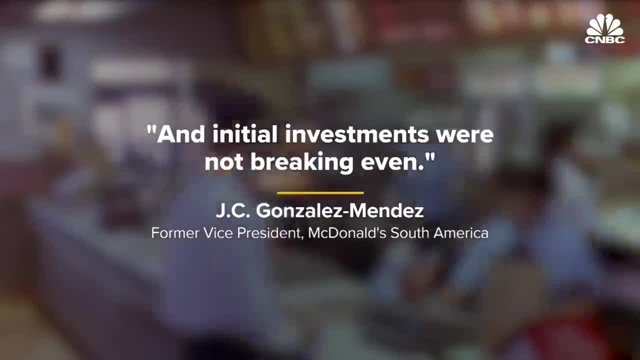 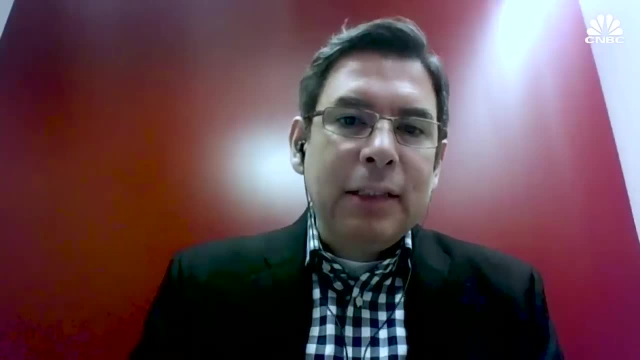 and initial investments were not breaking even. In the same year, McDonald's exited Bolivia. McDonald's also closed 700 stores down in nine other countries. So, from what I understand, McDonald's closed restaurants in Bolivia because they were underperforming relative to other places. 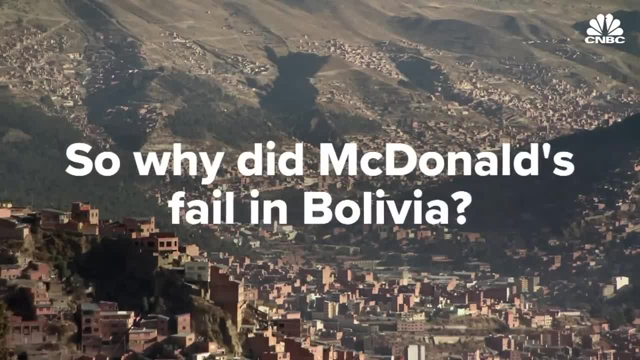 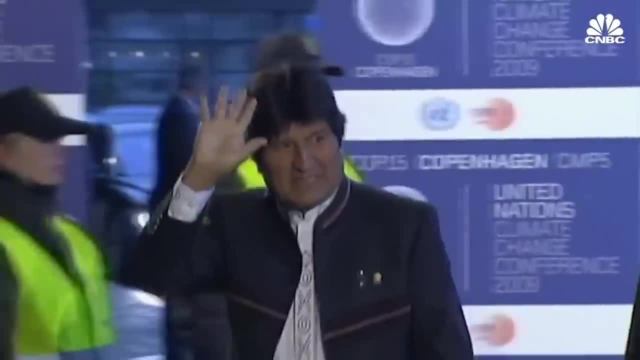 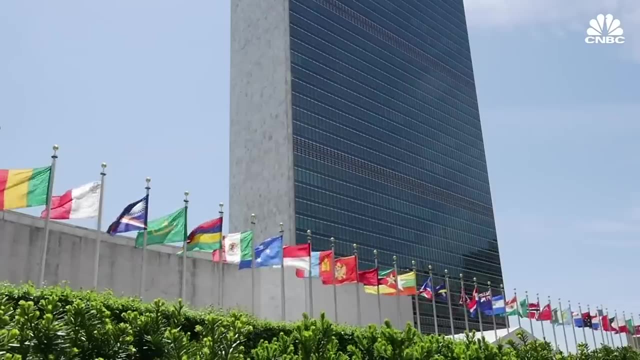 So why did McDonald's fail in Bolivia? Well, it's partly to do with the deep cultural rejection from Bolivia and its government. Although President Evo Morales was elected after McDonald's exit, his attitudes towards globalism reflected a long-held national sentiment. Back in February of 2013,, President Morales said this in a speech to the UN. 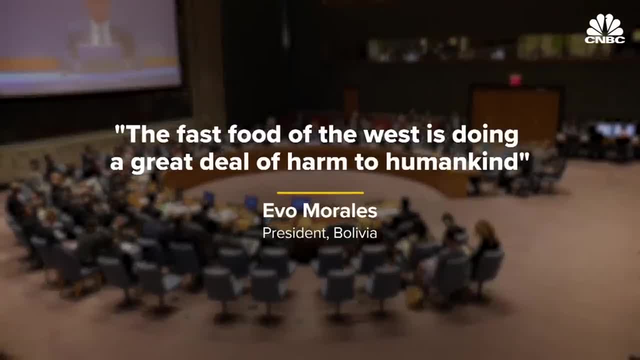 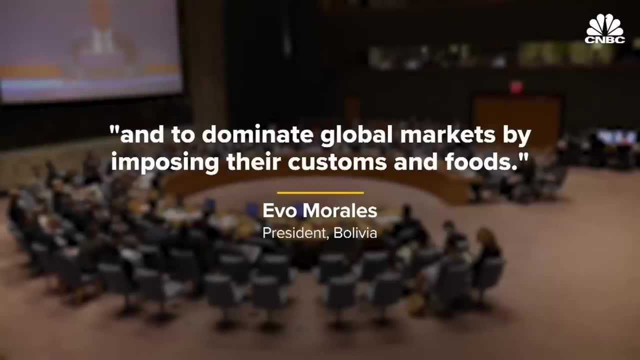 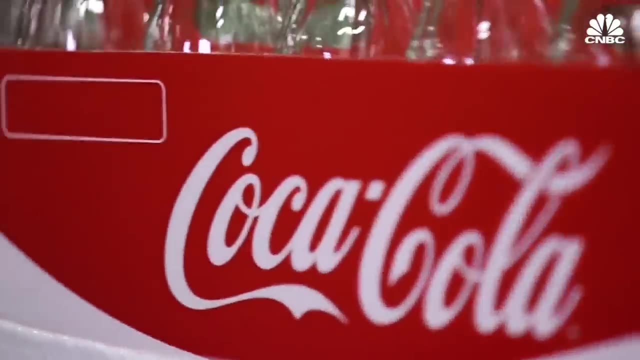 The fast food of the West is doing a great deal of harm to humankind, and the major multinational food companies seek to control the production of food and to dominate global markets by imposing their customs and foods. The president even banned the American staple and Bolivia Coca-Cola. In 2012,. Bolivia's president and the country's 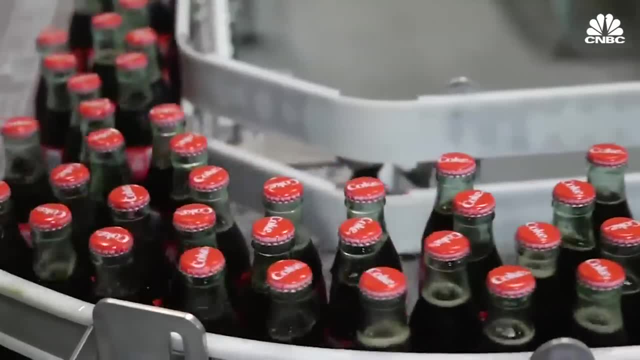 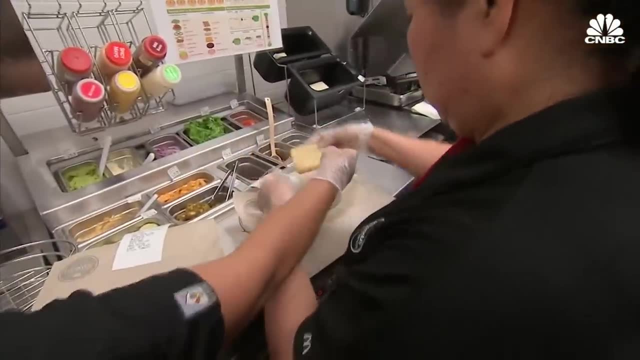 Minister of External Affairs announced the expulsion of Coca-Cola in Bolivia in favor of a traditional Bolivian drink. But it wasn't just politics that led to McDonald's demise. Bolivia's economy also played a role. Bolivia is one of South America's poorest countries. 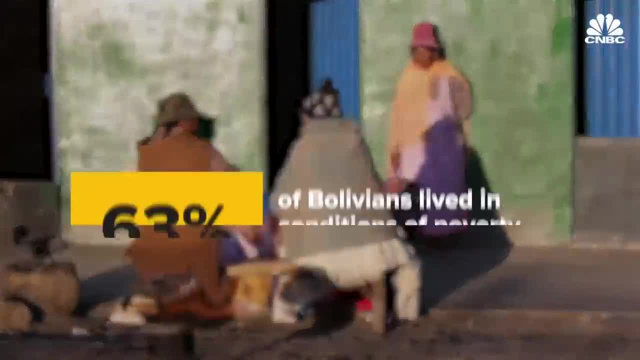 In 1997, when McDonald's first entered Bolivia, 63% Bolivians lived in conditions of poverty and 38 percent lived in extreme poverty. Bolivia's economy took a turn. Bolivia's economy was the worst economy on the planet, but its economy paid well. It helped make a difference to the environment. 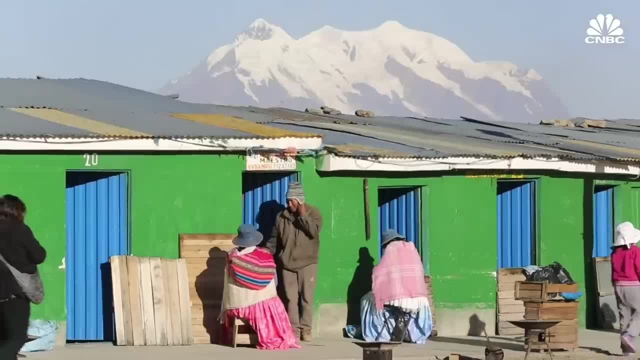 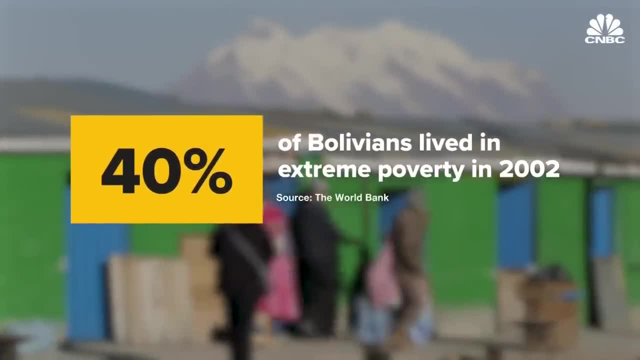